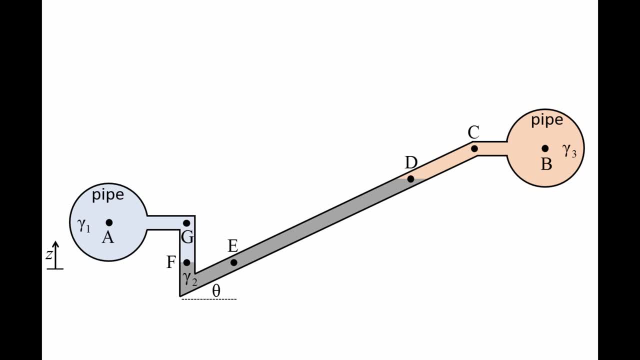 The specific weight of the fluid in the devices is gamma-1 and gamma-3,, while the gauge fluid has a specific weight of gamma-2.. Points A and B are at the center of the two sections of pipe. Point C is located at the same elevation as point B. 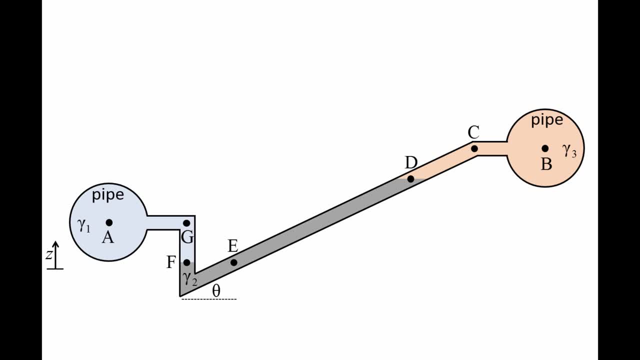 and point D is at the interface between fluids 2 and 3.. Point G is located at the same elevation as point A, and point F is at the interface between fluids 1 and 2.. The vertical distance between point A and the interface of fluids 1 and 2 is the height. 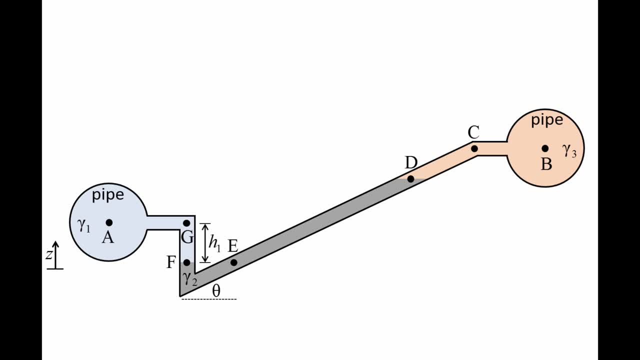 H1.. Point E is located at the same elevation as point F in the gauge fluid. The vertical distance between point B and the interface of fluids 2 and 3 is height H2.. The distance along the tube between points E and D is length L. 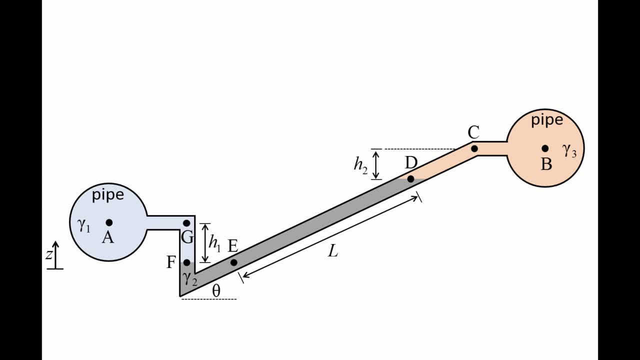 Now we will determine the pressure difference between points A and B using hydrostatic principles. We start at point B and will work our way around the manometer until we reach point A. The pressure at point B is Pb, And the pressure at point B is Pb. 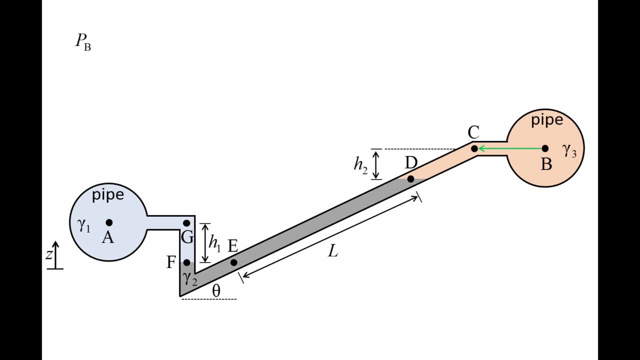 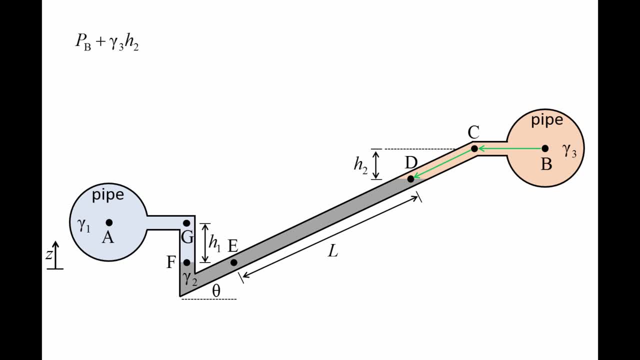 H2.. Notice that the distance between point C and D is longer than H2, but pressure only varies in the vertical direction. As we travel from point D to point E, the pressure increases by gamma 2 times the vertical component of L. 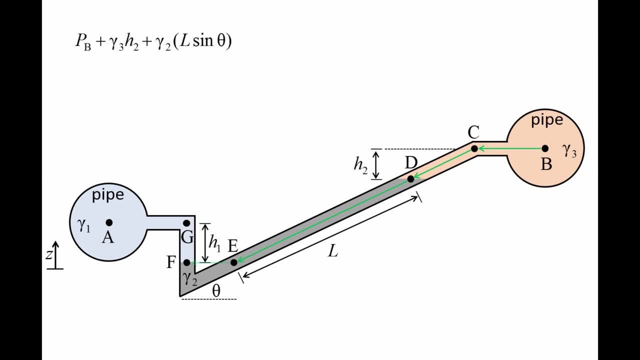 L times sine theta. We jump across to point F without a change in pressure, because points E and F are at the same elevation, then move to point G, while the pressure decreases by gamma 1 H1.. Finally, we move horizontally from point G to point A with no change in pressure. 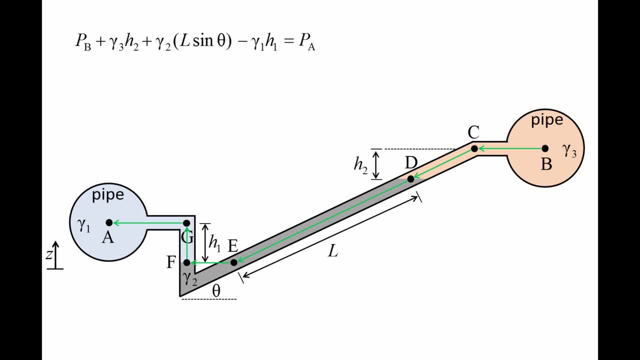 We have reached our destination and set the equation on the left equal to the pressure at point A. Rearranging the equation, we have an expression for the pressure difference. We add up this impression, which shows that we have calle WE and a varian.